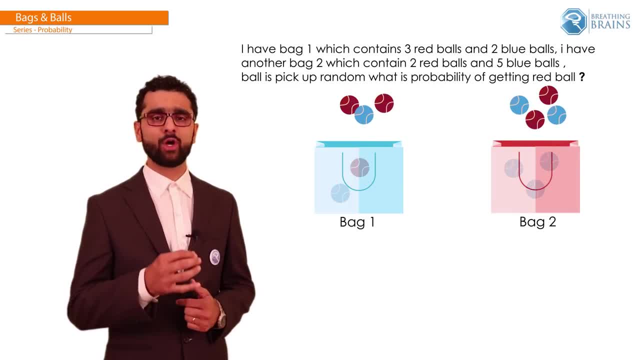 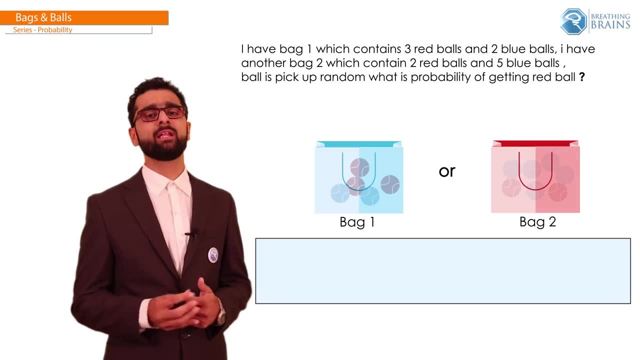 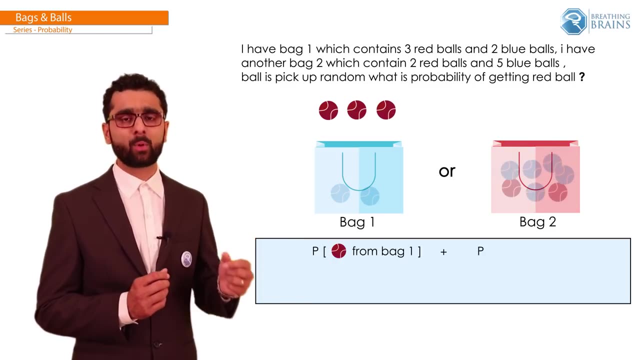 of getting a red ball Here. when I am drawing one ball, it can be either from bag 1 or from bag 2.. So the final answer will be probability of selecting a red ball from bag 1 or bag 4, which is plus probability of selecting a red ball from bag 2.. As we know, in the bag 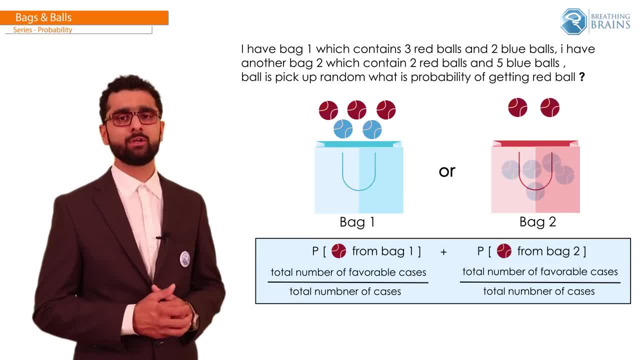 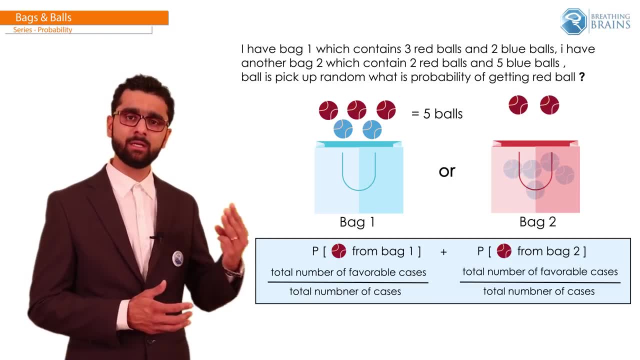 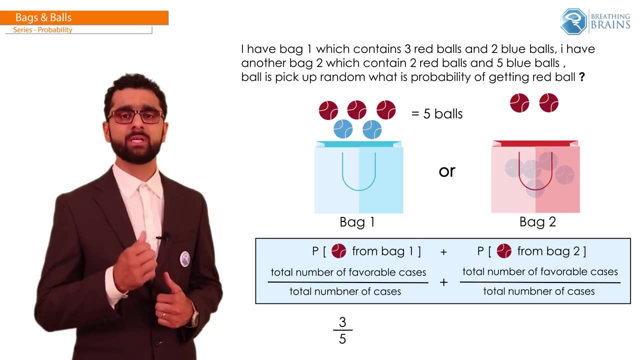 1, there are 3 red balls and 2 blue balls, So the total number of balls is 5, out of which one red ball is to be drawn, and hence favorable cases are 3.. So to draw one red ball from bag 1, the probability is 3 upon 5.. Similarly, for the second bag, the probability 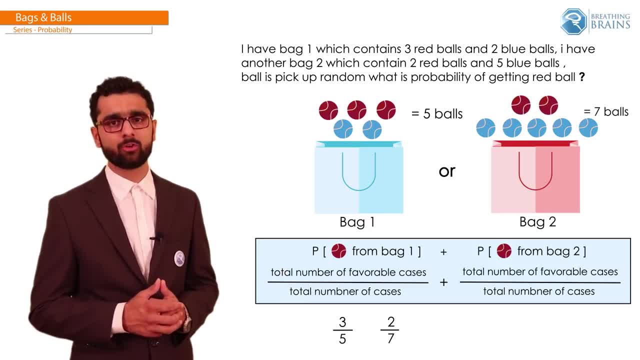 of a red ball is 2 upon 5.. So the final answer will be 3 upon 5, or, which is plus, 2 upon 7.. So when you calculate, you will get the final answer as 31 upon 35.. 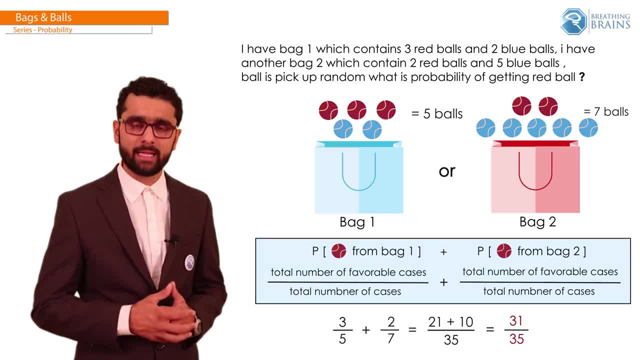 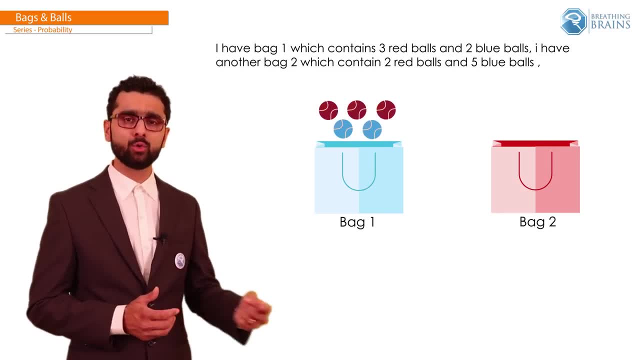 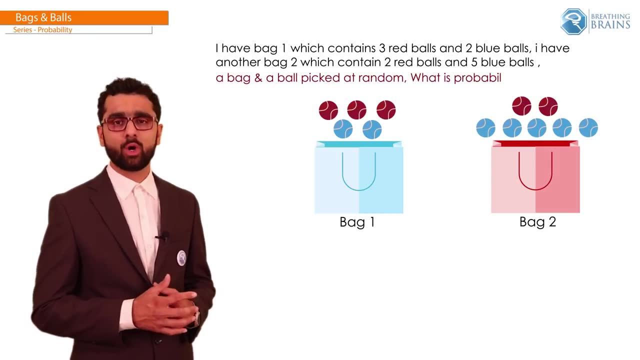 Now I will twist the question slightly In the same question, where bag 1 has 3 red and 2 blue balls and bag 2 has 2 red and 5 blue balls. Now a bag and a ball are picked at random. 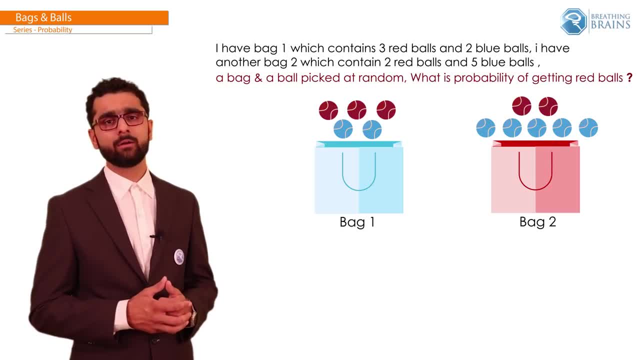 What is the probability of getting a red ball? Here we are first picking up the bag and then the ball, and hence we need to factor both the probabilities- probability of a bag and probability of the ball. So the final answer will be probability of selecting bag 1 from both the bags into probability. 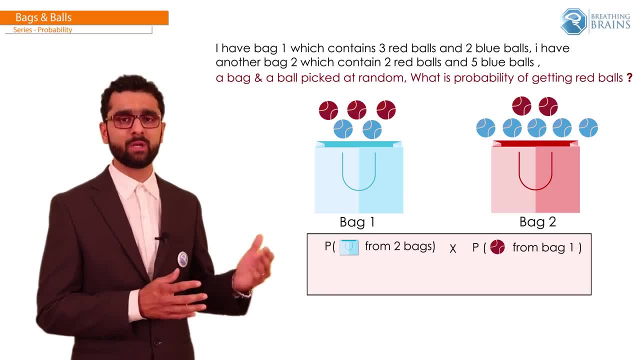 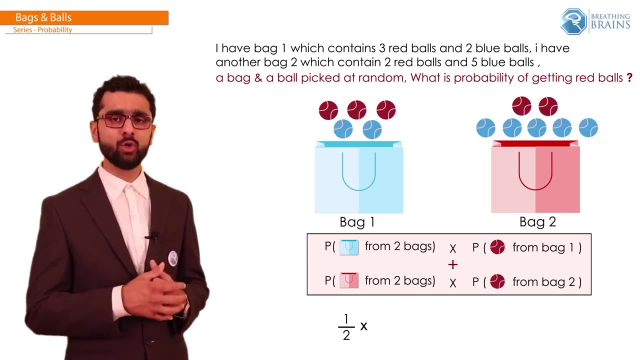 of red ball from bag 1 or, which is plus, probability of selecting the second bag from both the bags into probability of drawing the red ball from bag 2.. So to select bag 1 from 2 bags, we have 1 by 2 into to draw one red ball from bag 1. we have already seen. 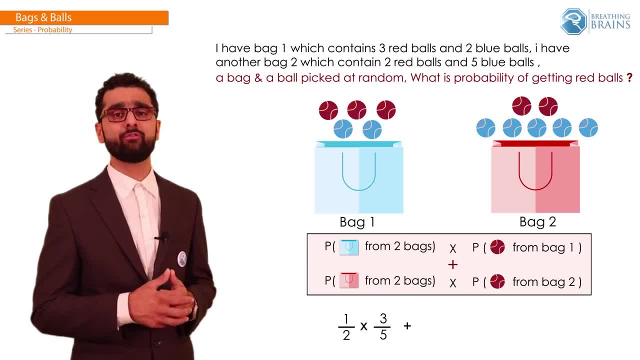 it is 3 upon 5. or to select the second bag from 2 bags, we have again 1 by 2. into. to select the red ball from bag 2, we have 2 by 7.. So when you calculate this you will get the final.